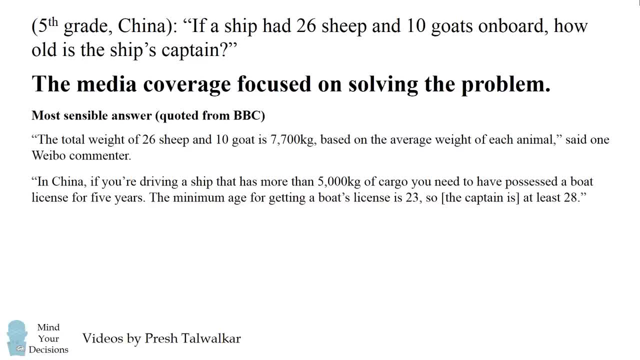 of cargo, you need to have possessed the following: You need to have a boat that has a boat license for at least five years. The minimum age for getting a boat's license is 23.. So the captain is at least 28.. That's a remarkable leap in logic. But if it sounds too crazy for you, 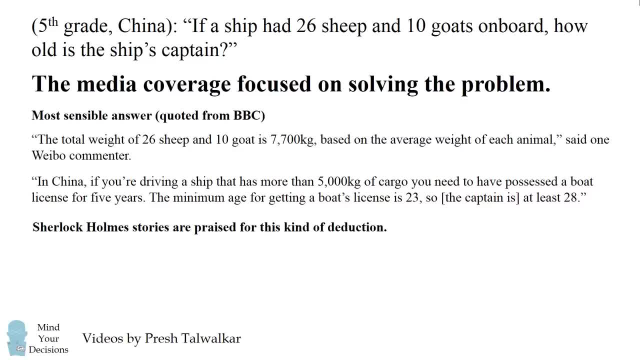 keep in mind that these kinds of deductions are very common in Sherlock Holmes stories. Take an example from The Hound of the Baskervilles. Sherlock Holmes deduces the man is under 30 years old, he's a family doctor and that he owns a dog. 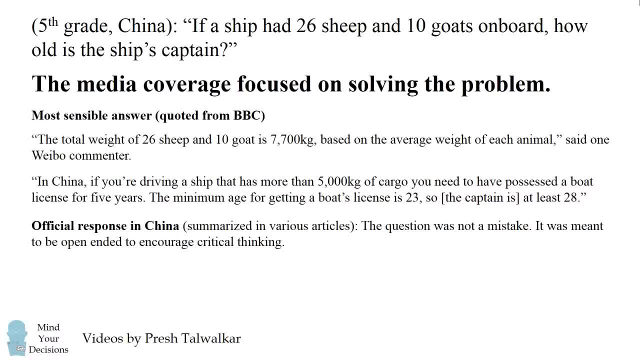 So the official response in China is that the question was not a mistake. It was actually meant to be open-ended and encourage critical thinking, which is usually not present in math class. That would be the end of the story, except this problem did not have its source. 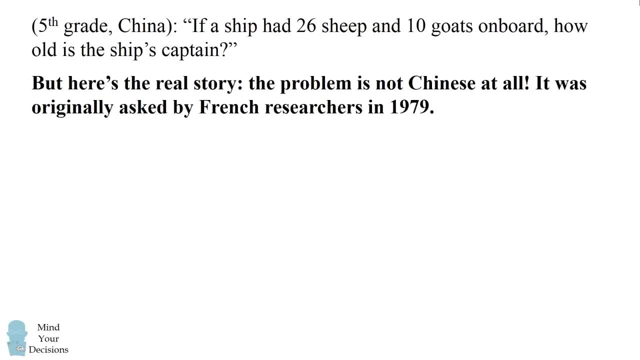 The real story is, the problem was originally asked by French researchers in 1979. This problem is nearly 40 years old. I learned about the problem's origin from Benjamin Dickman, who has a PhD in mathematics education from Columbia University. 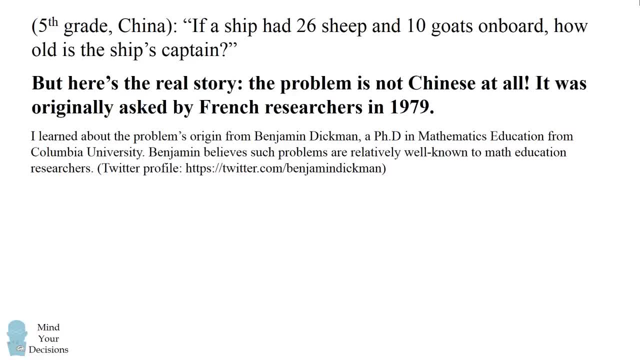 Benjamin heard about the problem because he believes that many people in math education have heard about this problem. He tweeted about it and you can check out his Twitter profile: twittercom slash: benjamin dickman. So from the sources that he tweeted and sent, we can actually find in 1979,. 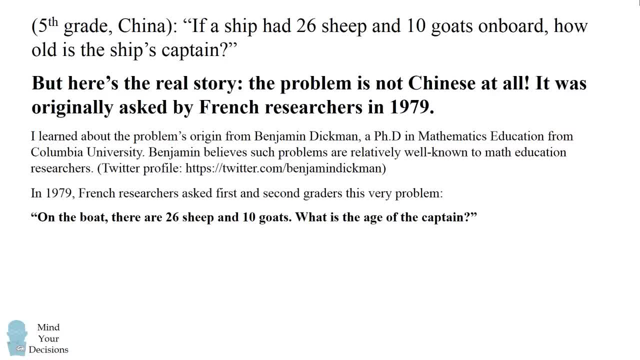 French researchers asked first and second graders the following problem: On the boat there are 26 sheep and 10 goats. What is the age of the captain? I couldn't believe it when I was seeing this. This problem has been asked nearly 40 years ago in almost exactly the same wording. 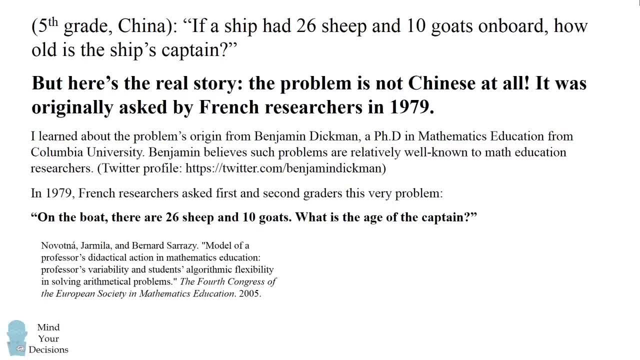 So what was the point of this exercise? Well, from reading some of these sources, the researchers had expected that most students would think the question is absurd. The correct answer would have to be: there is not enough information. But what they found was shocking. 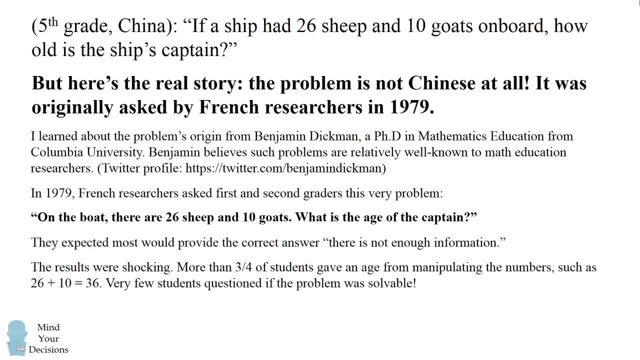 More than three-fourths of students actually tried to solve the problem by manipulating the numbers. They said something like: okay, the age must be 26 plus 10,, which equals 36.. Very few students questioned if the problem was even solvable. 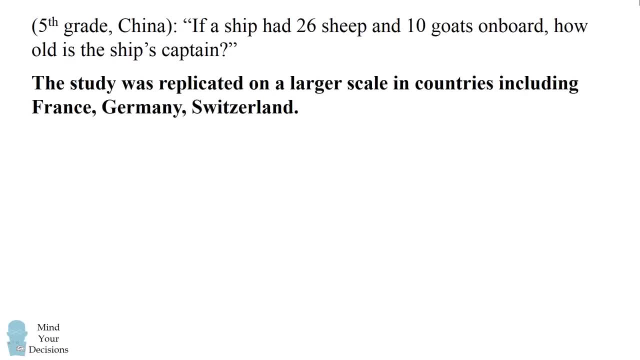 In fact, this was not just a fluke result. The study was replicated on a larger scale in countries including France, Germany and Switzerland, even by researchers from the University of New York. There were researchers who thought this was not even possible. 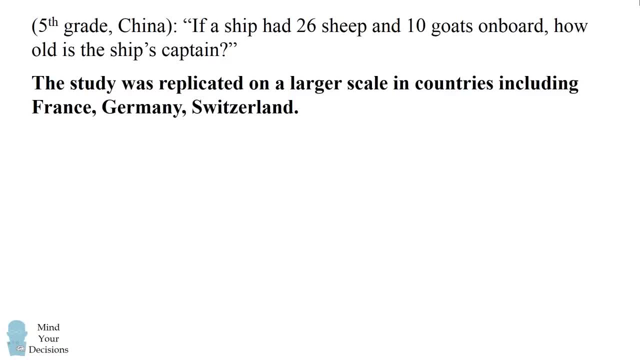 They were antagonistic to this hypothesis that students would just manipulate numbers, and they found the same thing. Gene Wierchenko emailed me about this related problem. His blog has math and logic problems, usually simpler than mine, and it has other posts. 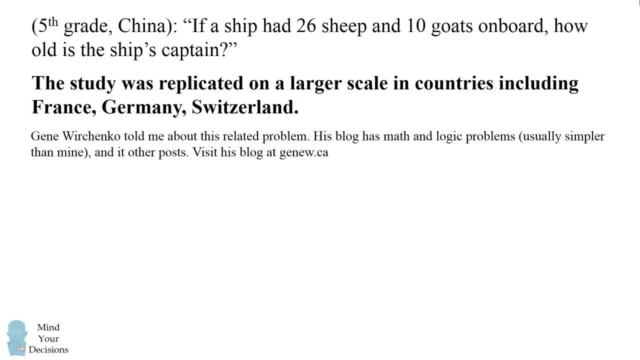 You can visit his blog at genewca. So the related question is the following: Gene Wierchenko's question is the following: There are 125 sheep and five dogs in a flock. How old is the shepherd? Well, once again, you would expect the correct answer. 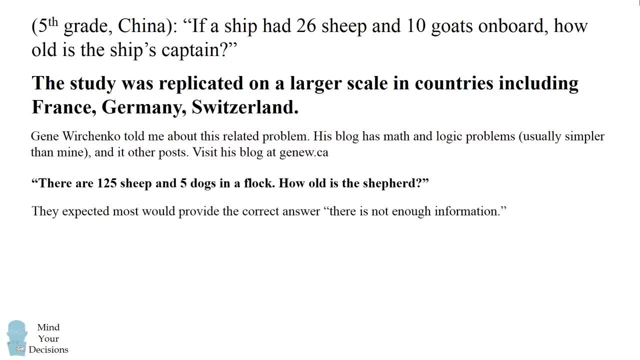 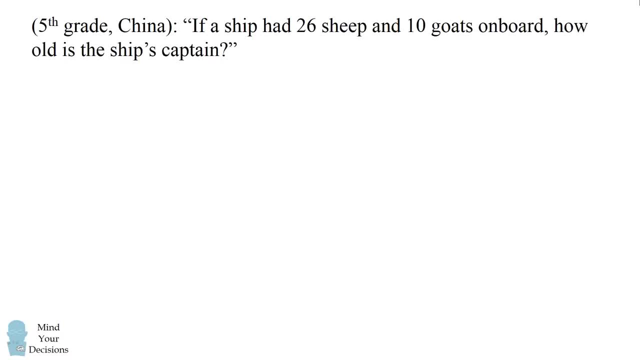 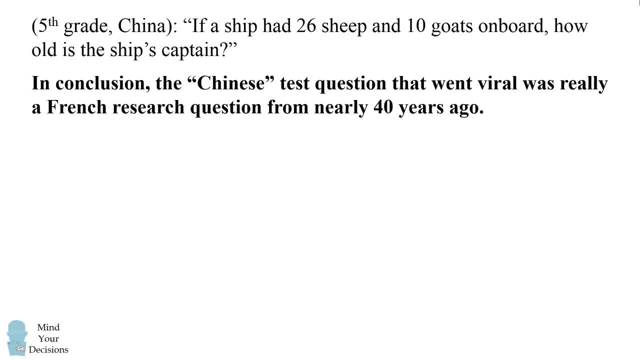 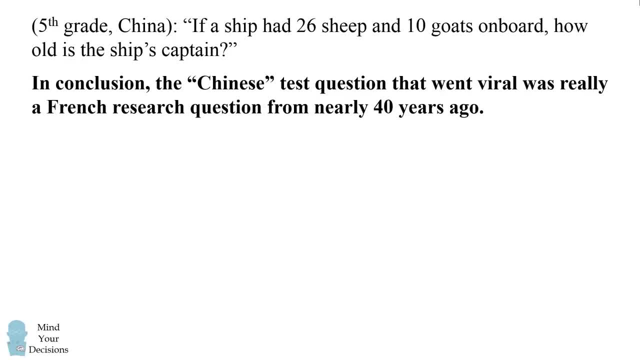 The so-called Chinese test question that went viral was really a French research question from nearly 40. that went viral was really a French research question from nearly 40 years ago. research question from nearly 40 years ago. research question from nearly 40 years ago. For such an absurd question. 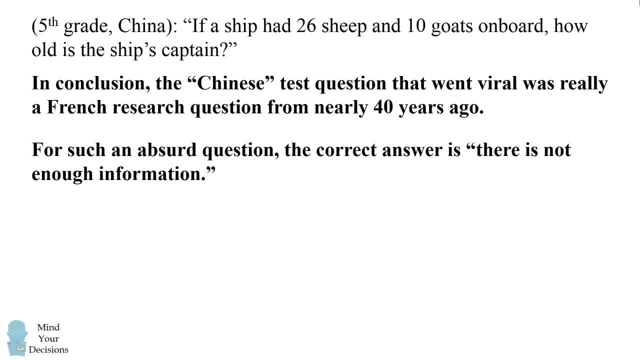 years ago For such an absurd question. years ago. For such an absurd question, the correct answer is that there is. For such an absurd question, the correct answer is that there is. For such an absurd question, the correct answer is that there is not enough information. the correct answer is that there is not enough information. the correct answer is that there is not enough information And I give credit to the school in not enough information, And I give credit to the school in not enough information, And I give credit to the school in China for asking this question. And I give credit to the school in China for asking this question And I give credit to the school in China for asking this question. We still need to improve the China for asking this question. We still need to improve the China for asking this question. We still need to improve the critical thinking skills of students. 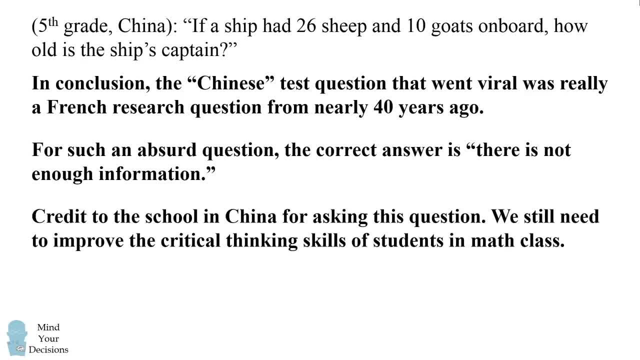 We still need to improve the critical thinking skills of students. We still need to improve the critical thinking skills of students in math class. We still keep critical thinking skills of students in math class. We still keep critical thinking skills of students in math class. We still keep thinking that every problem we get. in math class. We still keep thinking that every problem we get in math class. We still keep thinking that every problem we get is solvable. and it should be thinking that every problem we get is solvable. and it should be thinking that every problem we get is solvable and it should be solvable just by manipulating the. 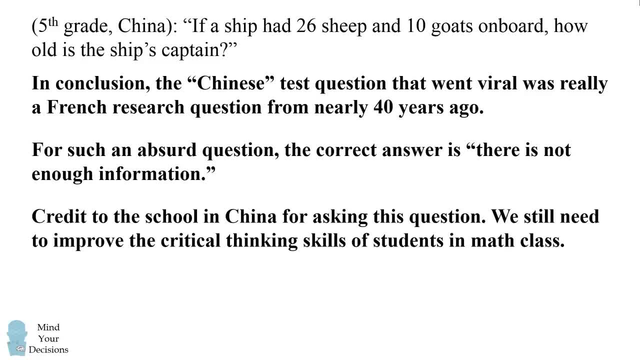 is solvable and it should be solvable just by manipulating the is solvable and it should be solvable just by manipulating the numbers we get. But we should solvable just by manipulating the numbers we get. But we should solvable just by manipulating the numbers we get. But we should always think: does the question? 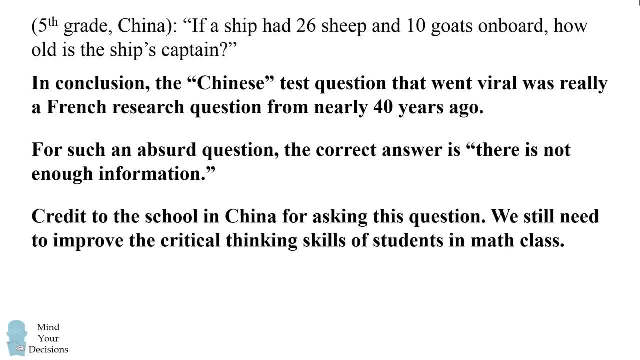 numbers we get. But we should always think: does the question? numbers we get, But we should always think: does the question actually make sense, Is there enough? always think: does the question actually make sense, Is there enough? always think: does the question actually make sense, Is there enough information to solve it? So that's. actually make sense. Is there enough information to solve it? So that's actually make sense. Is there enough information to solve it? So that's the real story to this viral math: information to solve it. So that's the real story to this viral math. information to solve it. So that's the real story to this viral math question from China. Thanks for the real story to this viral math question from China. Thanks for the real story to this viral math question from China. Thanks for watching this video Please. question from China. Thanks for watching this video. Please question from China. Thanks for watching this video. Please subscribe to my channel. I make watching this video. Please subscribe to my channel. I make watching this video. Please subscribe to my channel. I make videos on math. You can catch me on. subscribe to my channel. I make videos on math. You can catch me on. subscribe to my channel. I make videos on math. You can catch me on my blog. Mind Your Decisions If videos on math. You can catch me on my blog. Mind Your Decisions If. videos on math. You can catch me on my blog Mind Your Decisions If you like this video. you can my blog Mind Your Decisions If you like this video. you can my blog Mind Your Decisions If you like this video. you can check out my books, which are: